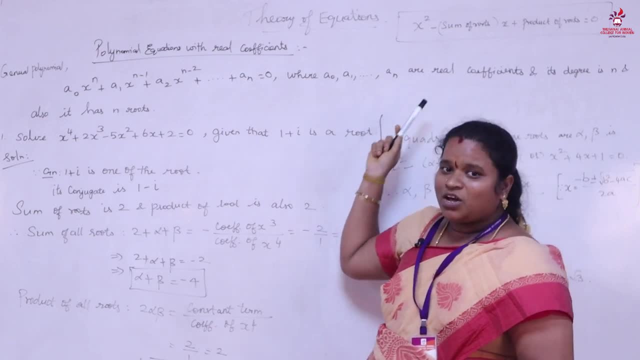 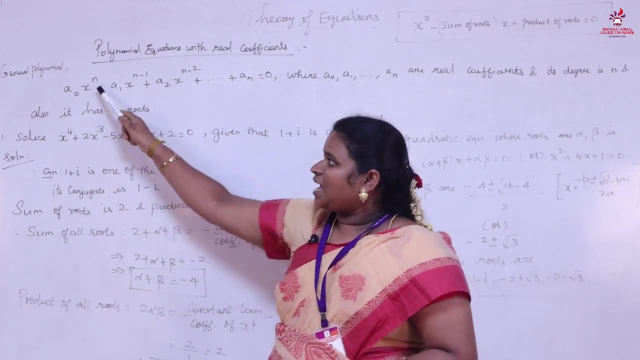 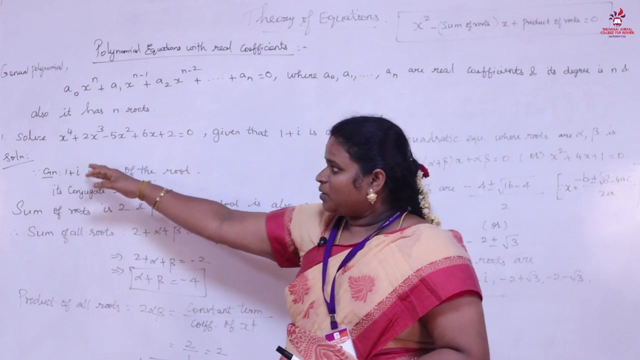 where a, naught, a, 1 a, 2, etc. up to a, n are said to be called as real coefficients and its degree will be n. and also it has n roots, because the highest degree of this equation will be n, so it has n roots. So let us we see some problem. So first problem is solved. 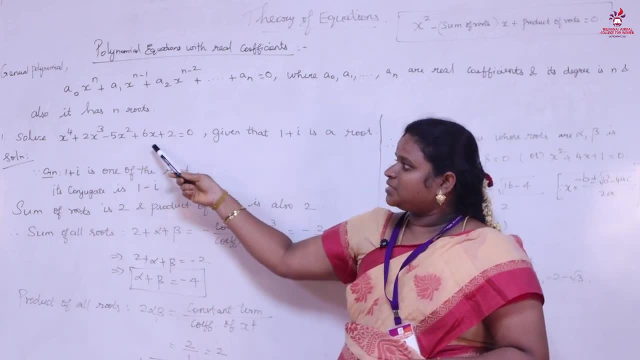 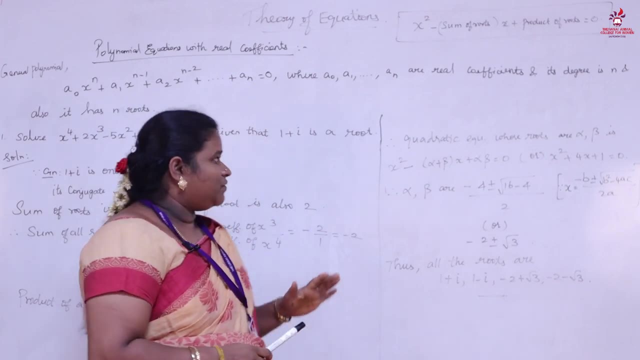 x power, 4 plus 2 x cube minus y x square plus 6 x plus 2, equal to 0.. And given that a condition- 1 plus i- is a root, this is a condition we have, they have given. So we need to find the roots of the equation. So how we need to find the roots of the equation. 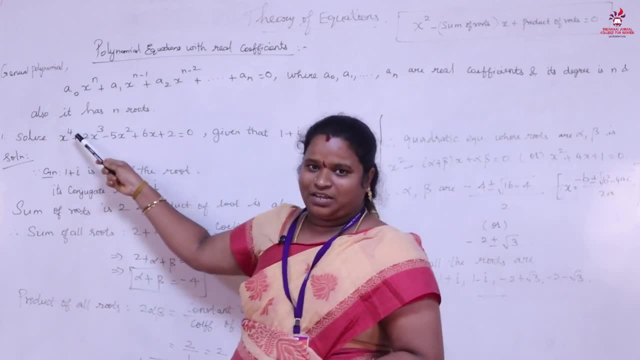 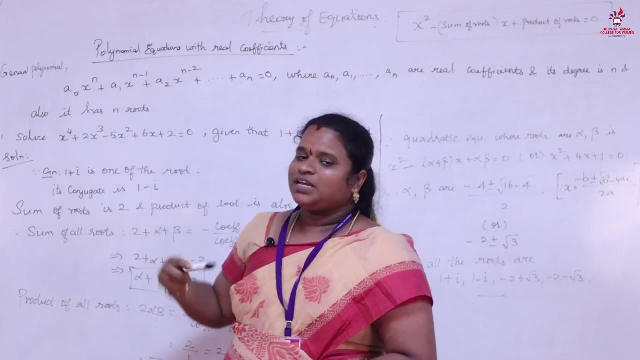 first we need to. so we need to find out the degree of the equation. the highest degree of the equation will be 4 here. So if the highest degree of equation will be 4 means we need 4 roots. but we have one root already in the equation itself, that is 1 plus i. So 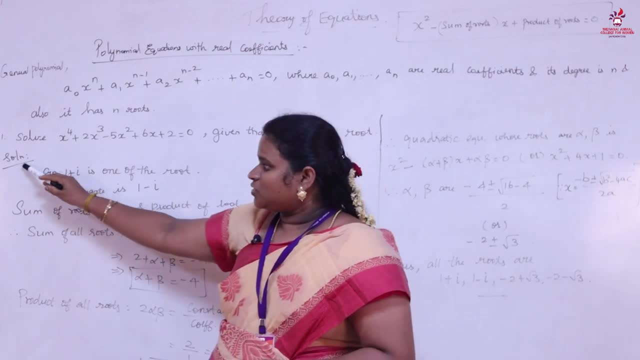 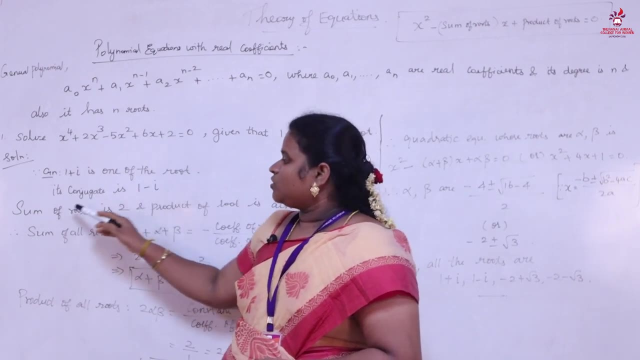 still we need 3 roots. to find it out The solution as given, 1 plus i, is one of the root, as in the question, So its conjugate is 1 minus i, So sum of roots and product of roots. we need to find it out. So in order. 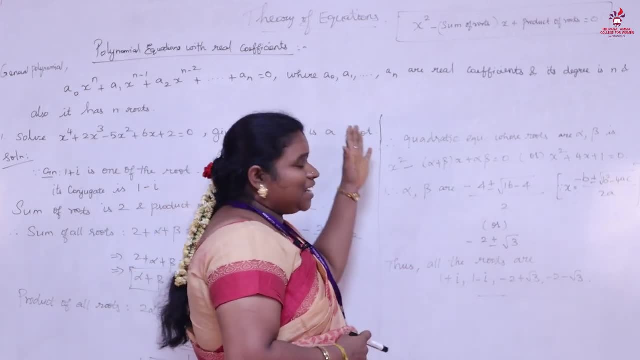 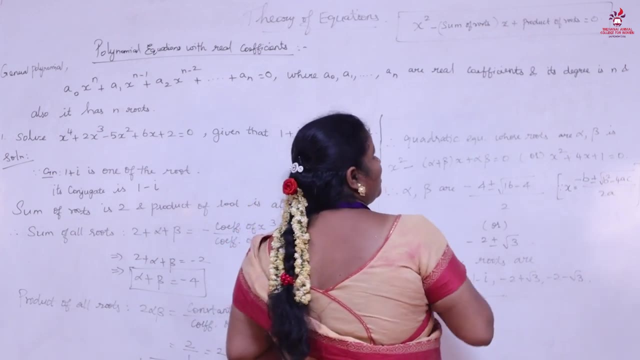 to find a sum of roots and product of root. So the general equation of the root will be x square minus sum of roots into x plus product of root equal to 0.. So in that we need to find sum of roots and product of roots First we need to find sum of roots. Sum of roots. 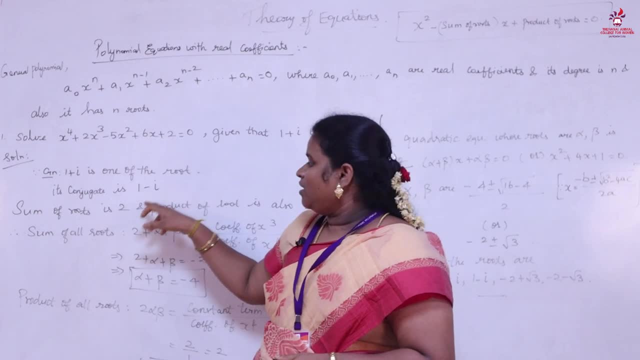 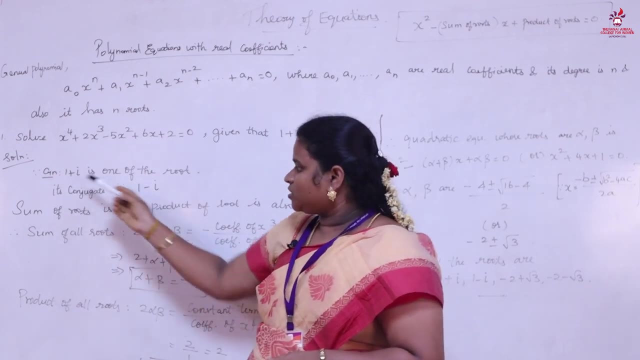 will be 1 plus i plus 1 minus x. So sum of roots will be 2 and product of root will be. we have to product these 2 roots, that is, 1 plus i as well as 1 minus i. If we product these 2 roots, we get 2.. So next we have to. 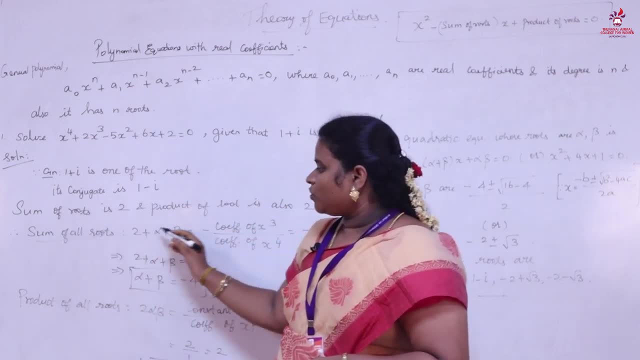 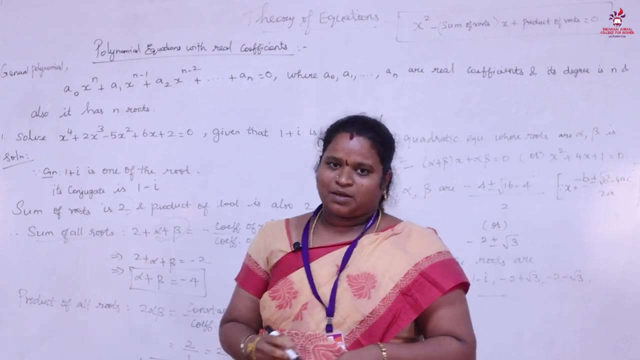 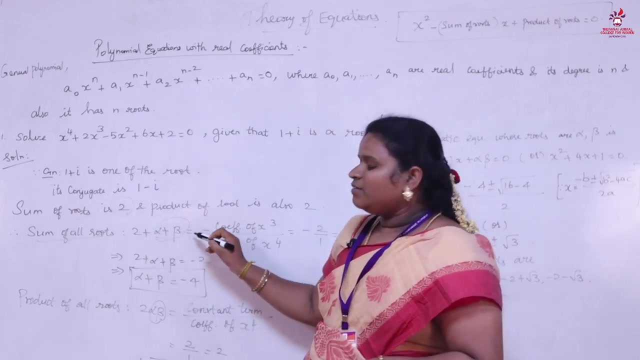 find sum of all roots and product of all roots. Sum of all roots would be: we have found that sum of roots is 2 and we know that alpha plus beta will be the sum of the root and alpha beta will be the product of the root. So sum of all roots equal to 2 plus alpha plus beta. 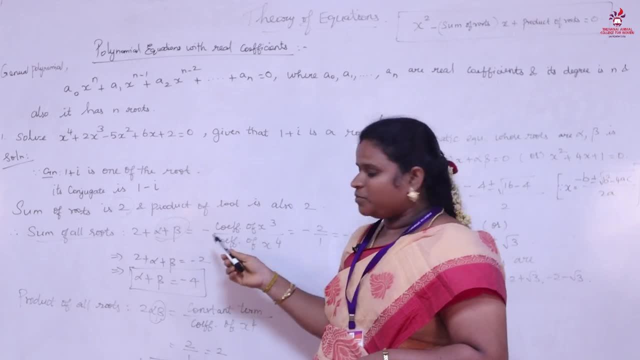 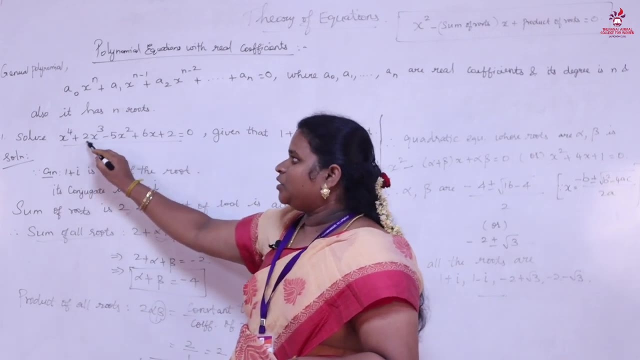 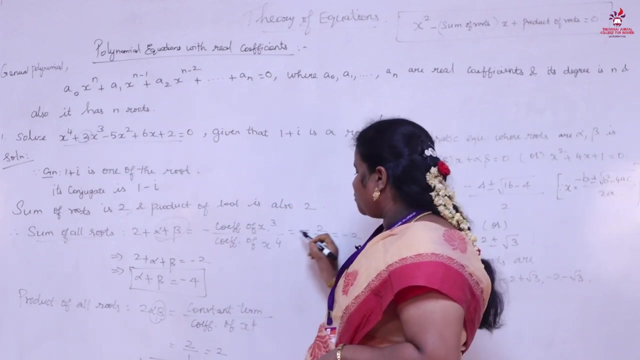 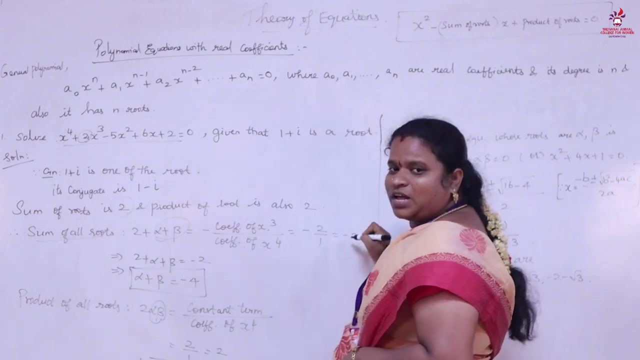 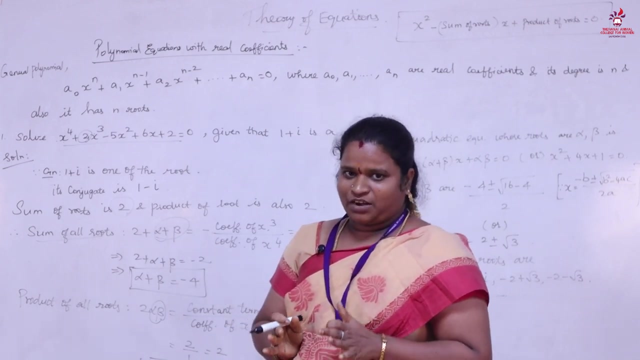 which is equal to 2 plus alpha plus beta, is equal to minus 2. means we need to find alpha plus beta, as well as alpha plus beta beta, First in case of sum of all roots means we need to find alpha plus beta equal to minus 2. 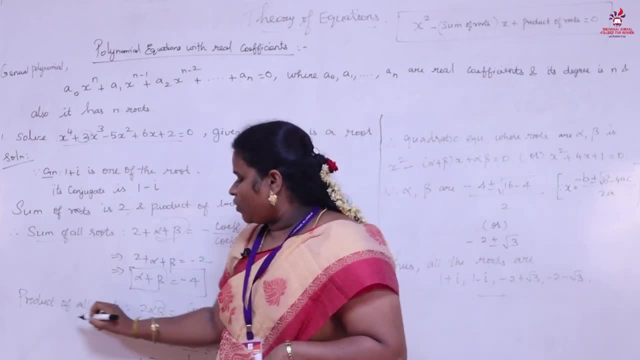 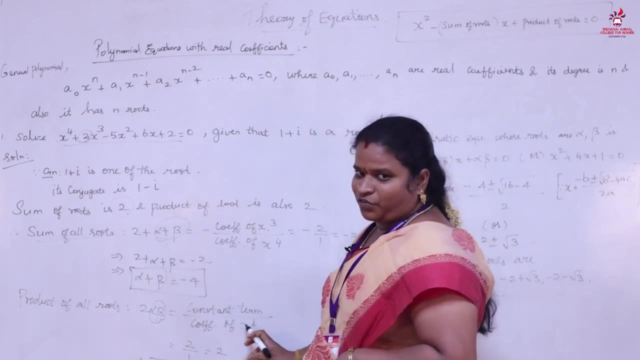 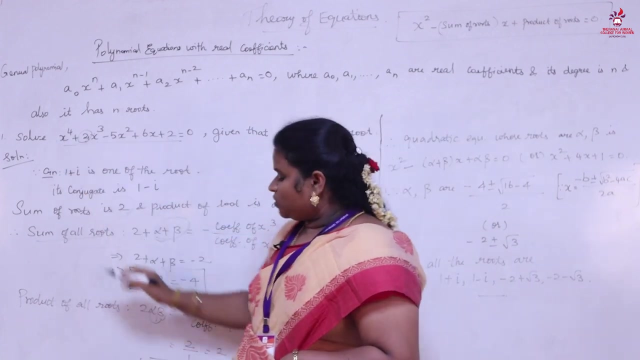 minus 2 will be minus 4.. Similarly, product of all roots will be 2. alpha beta is equal to the formula. will be constant term divided by coefficient of x power 4.. The constant term, the given question, is 2.. 2 divided by coefficient of x power, 4 will be 1.. So we have to substitute the value and we 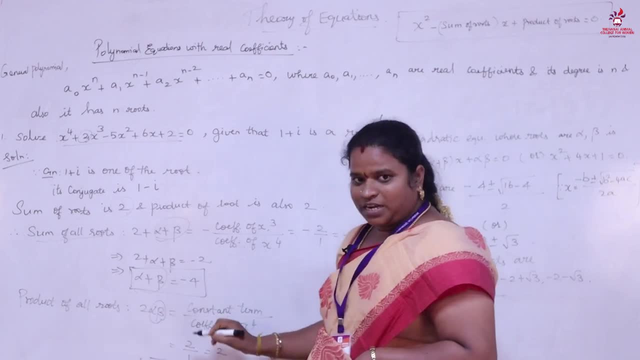 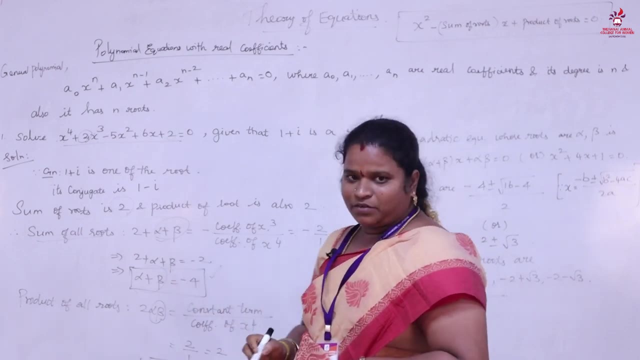 get the answer as 2.. So 2 alpha beta equal to 2 means we need alpha beta alone, So the value will be 1.. If we found alpha plus beta equal to minus 4 and alpha beta equal to 1 means at last we need 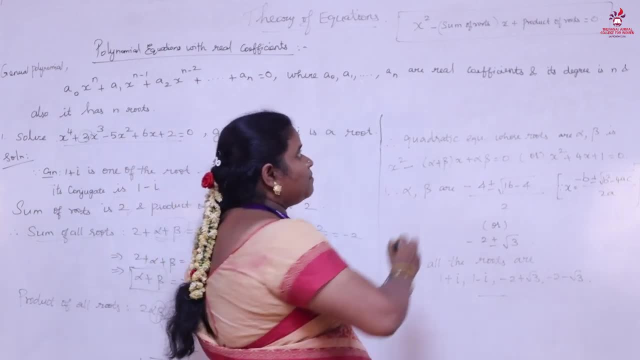 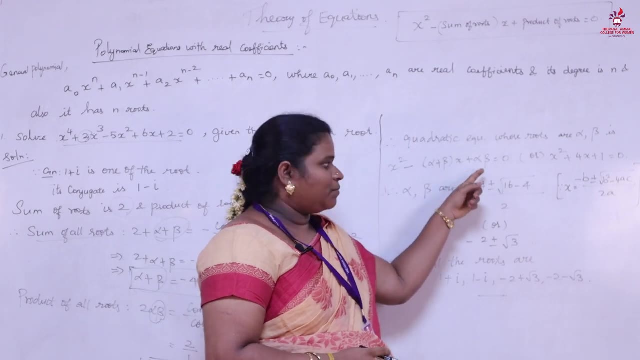 to find the quadratic equation. The solution will be: x square minus sum of roots into x plus product of root equal to 0. that is, x square minus alpha plus beta into x plus alpha beta equal to 0.. We found alpha plus beta equal to minus 4 here and alpha beta equal to 1.. So we just 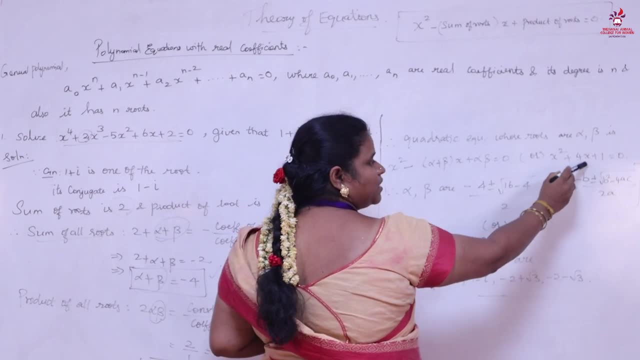 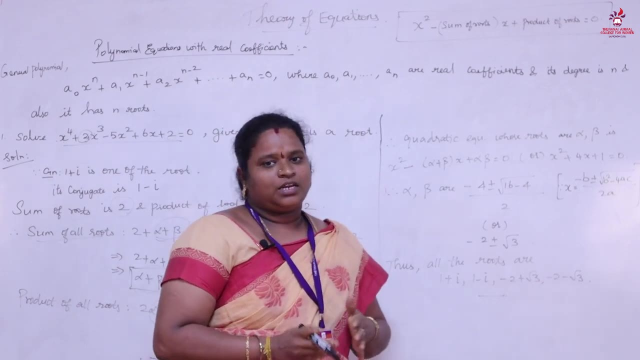 substitute The values here, so we get x power. x square plus 4x plus 1 is equal to 0.. So at last we need to find the roots. We have one root in the question, So still, we need to find three more roots. So for: 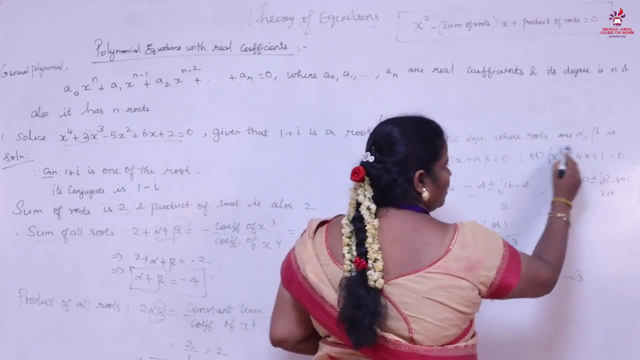 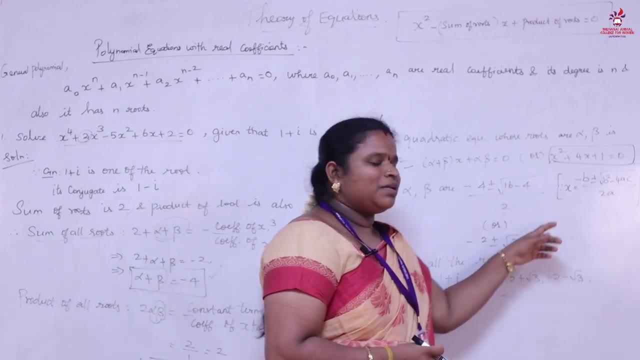 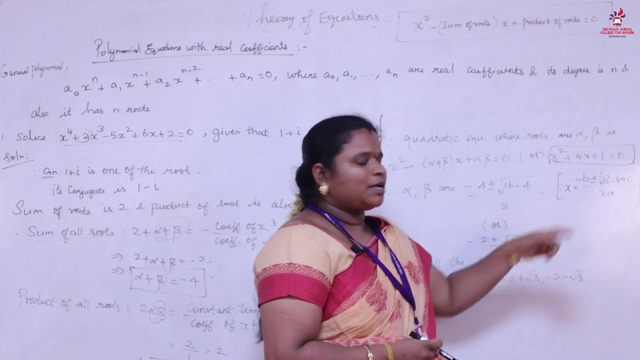 that alpha beta root will be. so we have to solve this equation. In normal i method we can't solve the equation because we can't get the root, So by using formula method. the formula method will be: x is equal to minus b, plus or minus square root of b square minus 4ac by 2a. Here we have to. 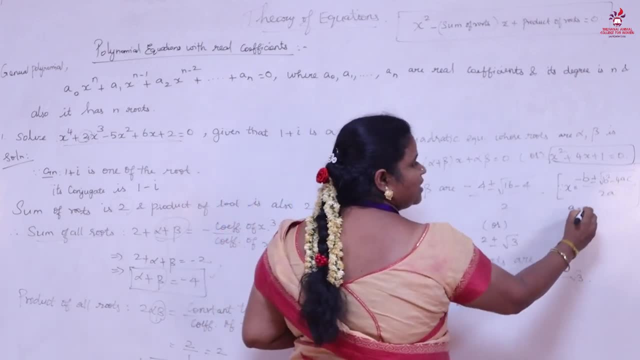 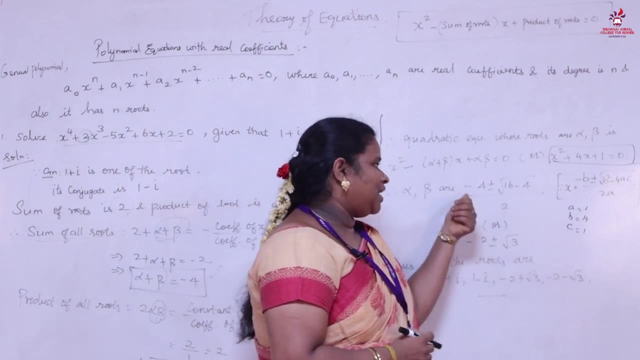 substitute. So in this equation a is to be considered as 1 and b is to be considered as 4 and c is to be considered as 1.. So we have to substitute these values and we get minus, 4, plus or minus root of. 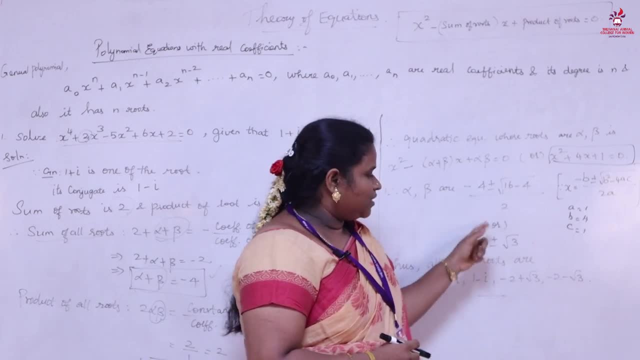 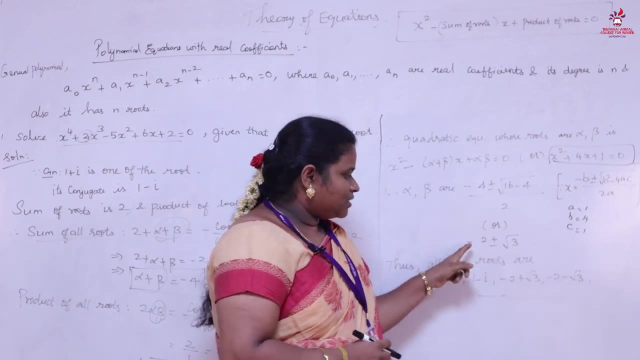 16 minus 4 by 2, and after we simplify this we get minus 2 plus or minus root 3.. So at last plus or minus root 3 means we get two roots, That is, one is minus 2 plus root 3 and another one root is.